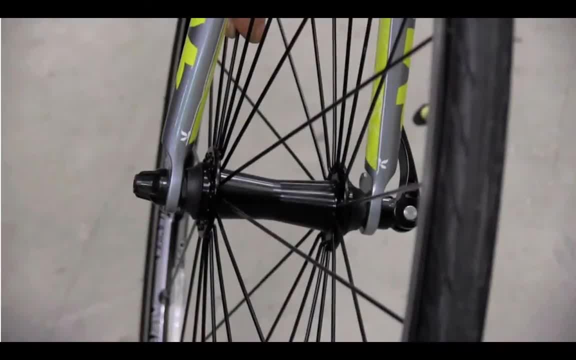 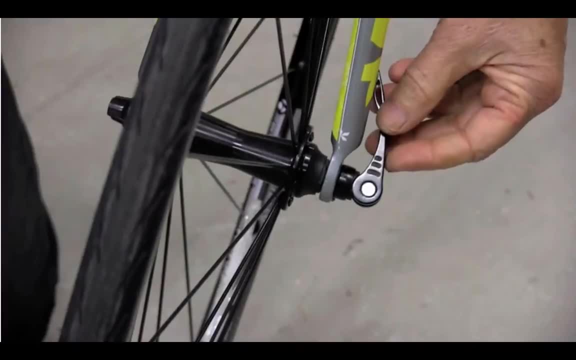 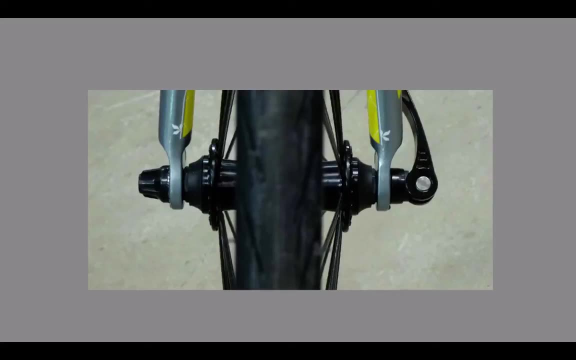 are closed and locked. My front wheel is safely installed in the front fork And the skewer here is tightly closed. Here is a close up of my front wheel with the skewer closed. This line is the center of the skewer. That's an extension to it. 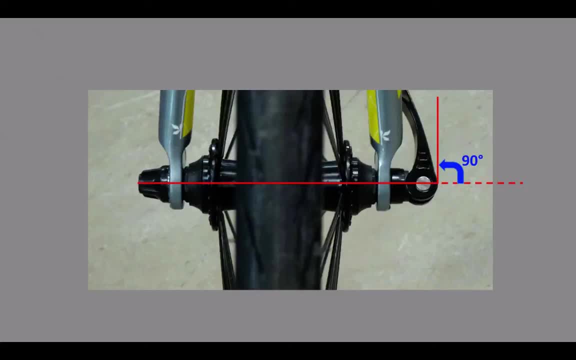 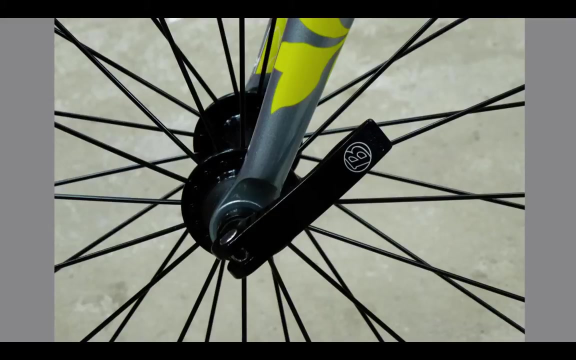 That's a perpendicular line. Therefore, that's a 90 degree angle. Ideally, I want my skewer to be more like that, Which would be more than a 90 degree angle. A good place to tuck the skewer lever in is right behind the front fork. 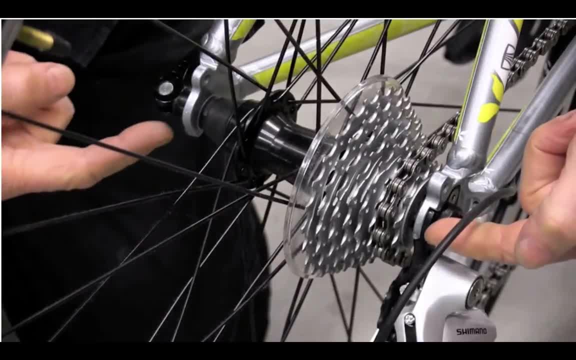 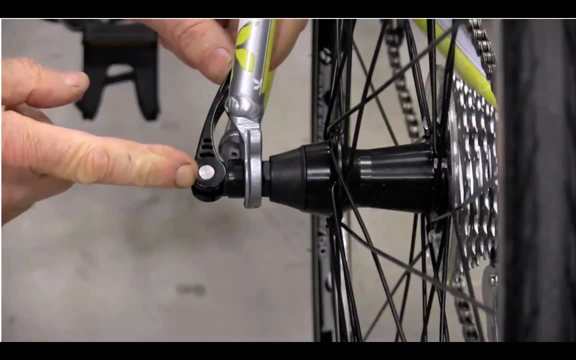 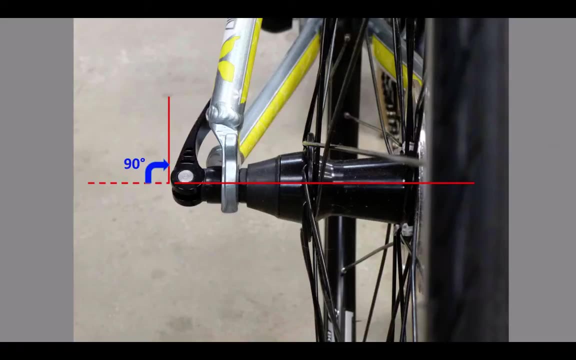 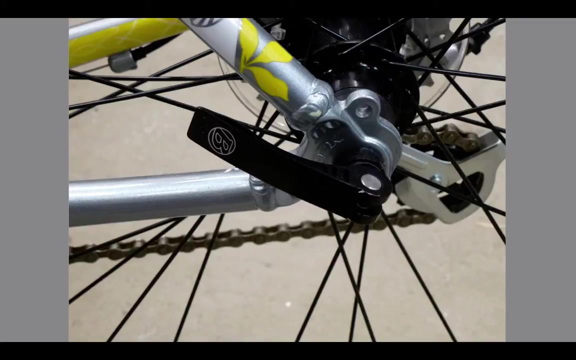 The rear wheel is securely installed between my dropouts And once again, my skewer is tightly closed. Here again I've closed the skewer And now I'm going to close it. The rear lever is at the center of my brake lever. 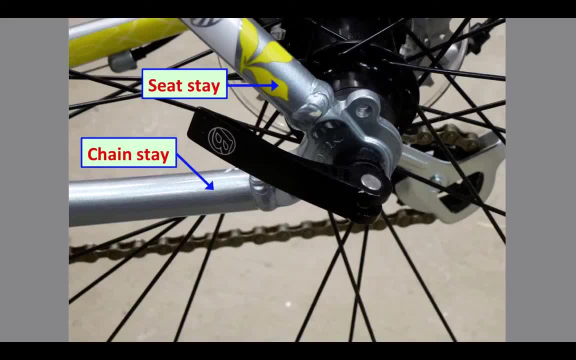 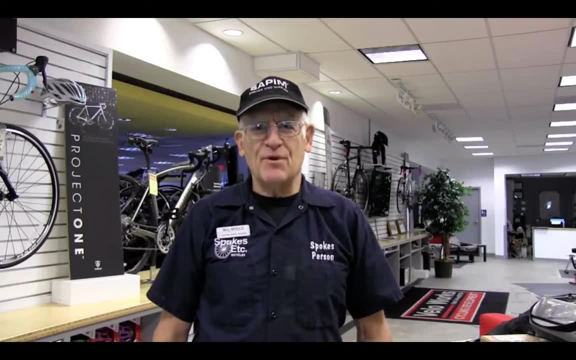 And it's tightly closed. Here is another example. I want to make sure that the wheels are properly installed in the front fork And that the front fork is completely closed. Here is another example. Here is my rear skewer lever in place. 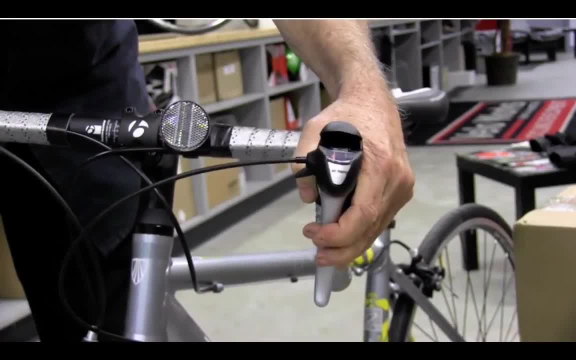 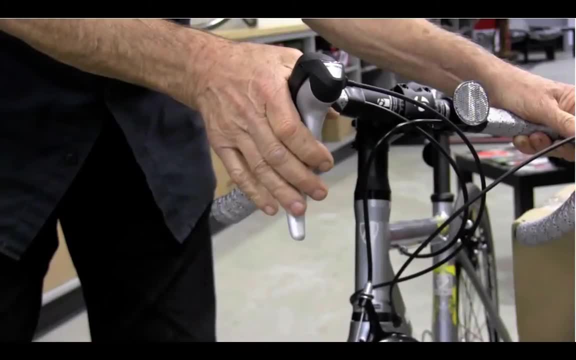 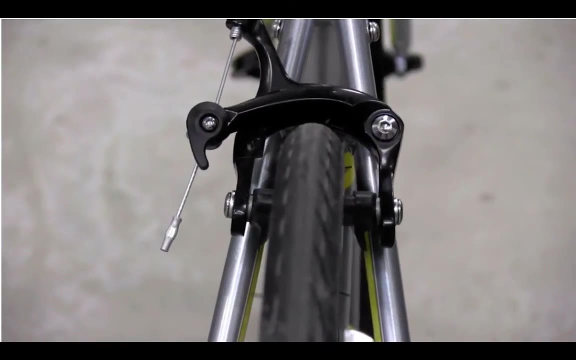 When I'm adding a brake lever, I'm going to make sure that the front brake lever is close behind the front fork. Where I have my brake lever, brake closes And when I squeeze the lever on the rear brake, the rear brake closes. 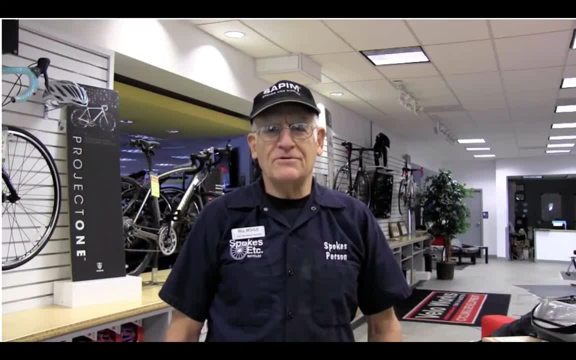 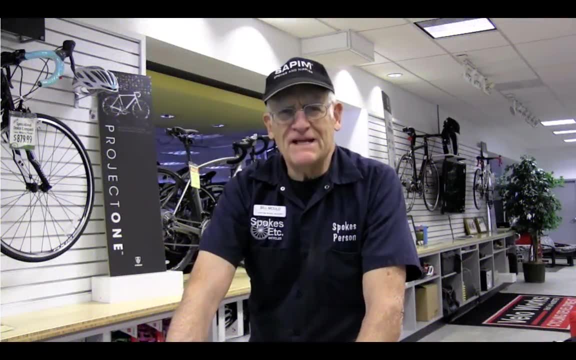 I also want to make sure that the handlebars are connected to the front wheel. Let me show you what I mean. The situation I'm going to show you now is about as dangerous as it can get when you're riding your bicycle And it occurs. 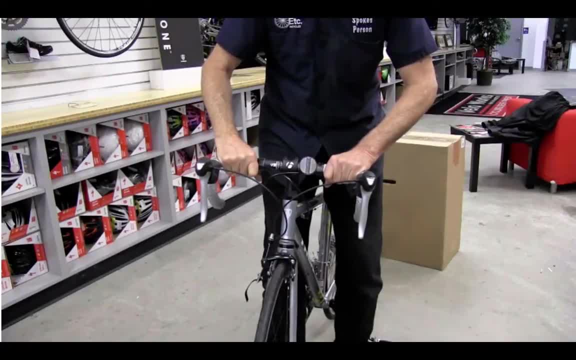 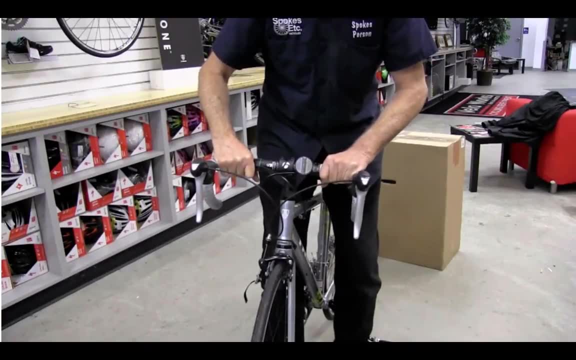 when the handlebars are not connected to the front fork and the wheel so that as you turn the handlebars, the wheel doesn't turn with the handlebars. That means you have no steering. We're going to focus on this part of the bike right. 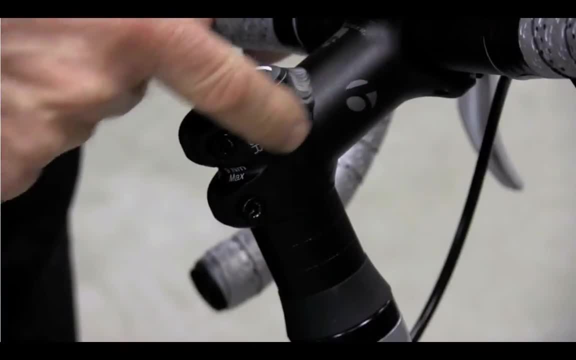 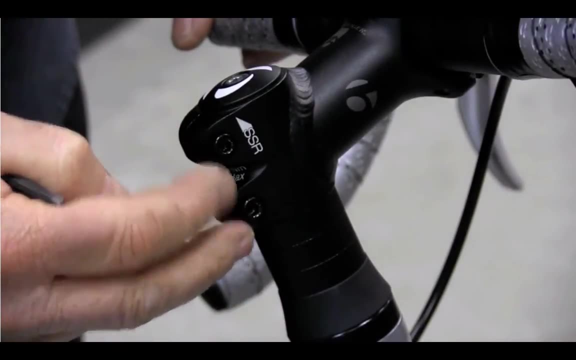 here. This piece here is the stem, and the stem is what connects the handlebars to the fork. These two bolts here on the stem have to be tight. If these bolts are loose then the handlebars are not connected to the fork and the handlebars are not connected to the fork.